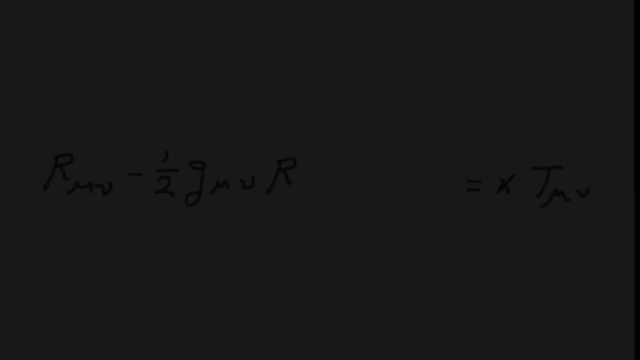 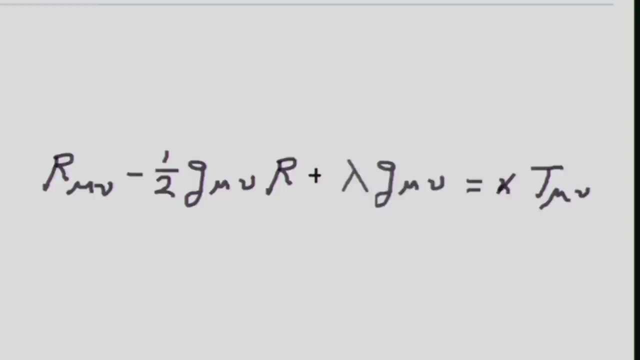 These equations you've seen before, they're Einstein's field equations. You all know that Einstein realized that you could put another term into the equations, the cosmological term, And that's solving a parameter lambda, And of course he put it on the left side. 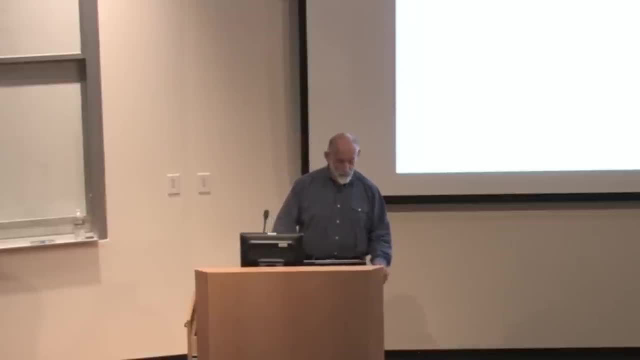 The left side has to do with geometry, the right side has to do with energy and momentum, the sources of the gravitational field. But it didn't take long and in particular the conversation between Pauli and Dirac had to do with the idea of putting it on the other side of the equation. 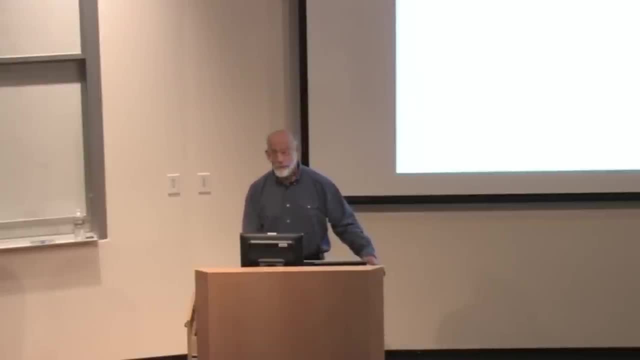 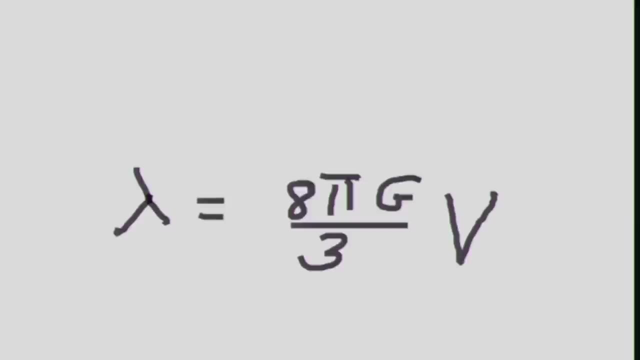 On the other side of the equation, the cosmological constant becomes part of the source And we give it the name of the equation. We give it the name vacuum energy, V for vacuum. it could also be V for potential energy, but V for vacuum energy. and we understand today that a vacuum energy could be the source- and not only could be but should be the source- of the accelerated expansion of the universe. 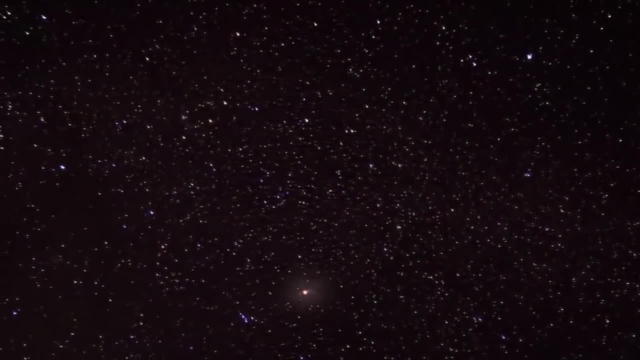 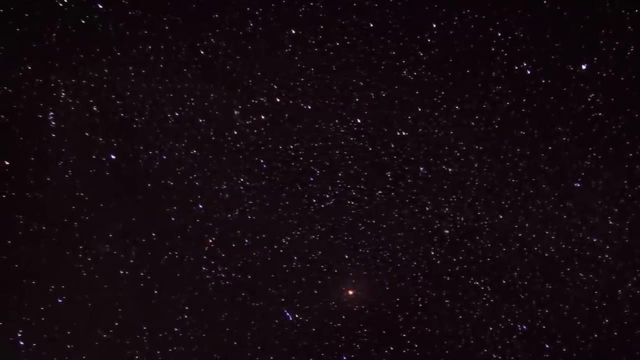 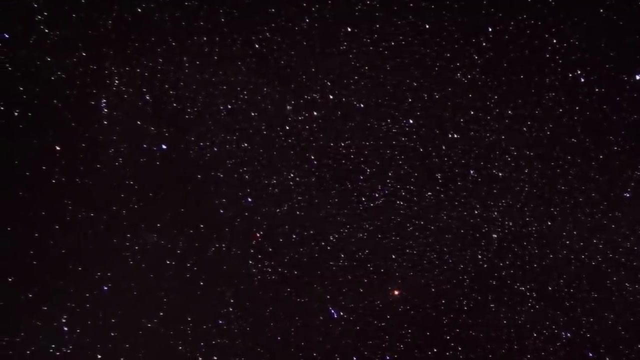 What is surprising about the existence of a cosmological constant? Nothing is surprising about the existence of a cosmological constant, as I'll explain. What is surprising, and very surprising, is how little dark energy there is. Not that there is dark energy. 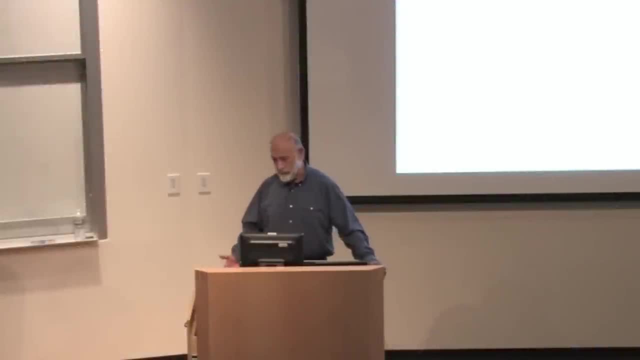 The press gets it all wrong. They say: what is this mysterious dark energy? The real question is: why is this mysterious dark energy so very, very small? Okay, let's just review for a moment. Okay, let's just review for a moment. 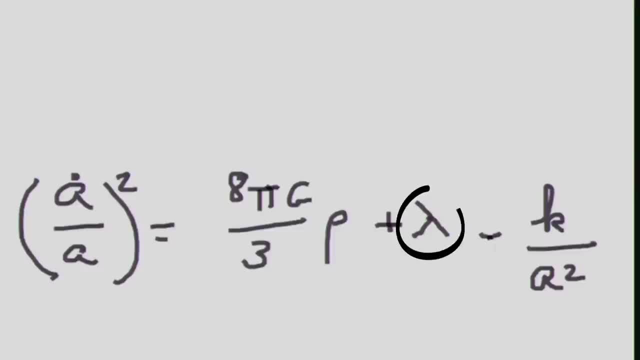 What dark energy does lambda? lambda meaning the cosmological constant dark energy, vacuum energy, all the same stuff. First of all, it enters into Einstein's field equations which, for a simple cosmology, FRW cosmology- is just the standard FRW equations with lambda on the right side. 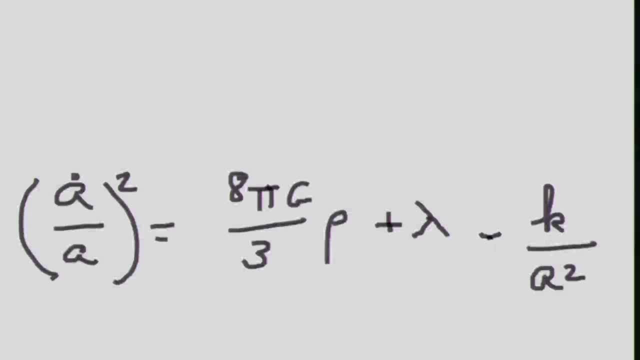 As you know- I'm sure most of you know or all of you know- that the energy density term, rho, for ordinary sources of energy doesn't matter. canon zero, The only term. the term decreases the cosmological constant term and so it dominates when the universe gets big. 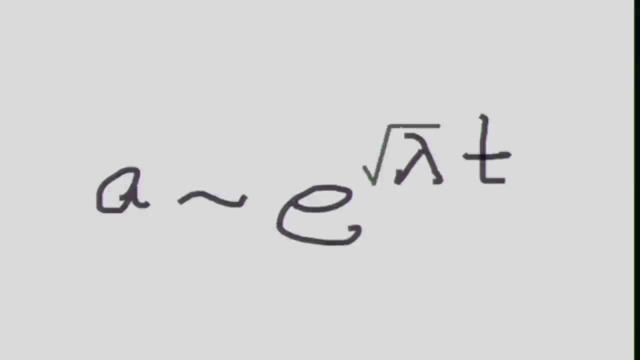 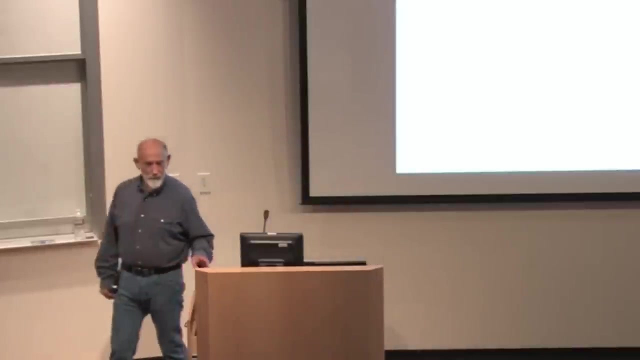 You can throw everything else away, solve the equation, and what do you get? You get exponential expansion, And so the existence of a dark energy should imply an exponential expansion and exponential expansion. in fact, the first i heard of the problem came from david finkelstein sometime. 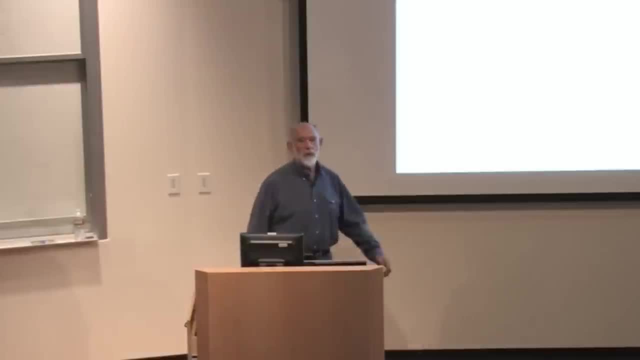 around nineteen, sixty seven. he explained to me that if you took all the dark energy or all vacuum energy that comes from scales up to about the electron mass, the vacuum energy- he didn't call it cosmological constant- the vacuum energy would be such that its gravitational effects would curl the universe up into nothing much. 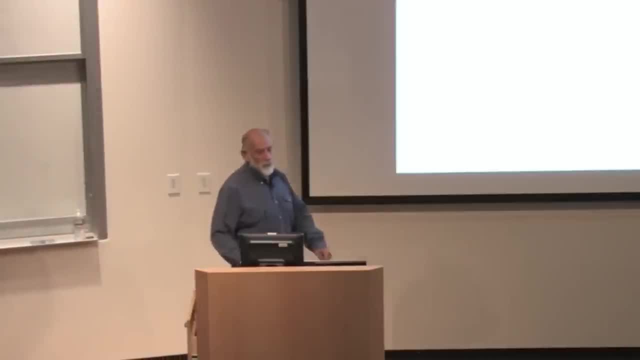 bigger. i can't remember if he said the orbit of the moon or the size of the moon. this is something we could work out, but a very small universe. so we have a puzzle. now let's take a theorist's view of it. theorist's view of it. 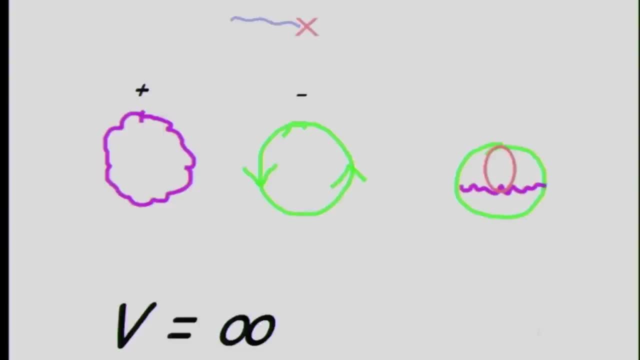 is that vacuum energy- putting lambda on the right hand side- comes from various quantum field theory processes. the first kind of process is basically classical. it could come from any sources of classical vacuum energy, classical, uh, whatever, whatever it happens to be a bare cosmological constant, a field potential, whatever you like. 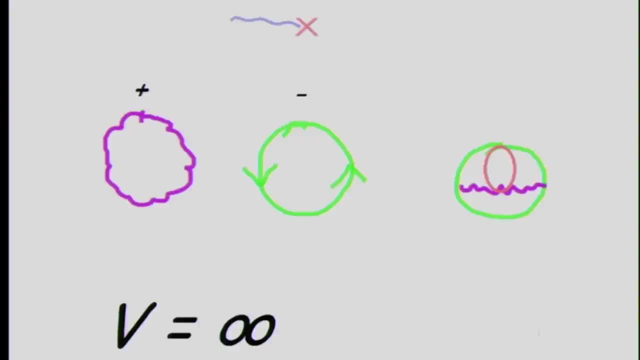 no loops in it, no quantum mechanics. but whatever it is, there are corrections to it, radiative corrections, feynman diagrams, and the problem is, as dirac correctly perceived, these feynman diagrams are all infinite. so the vacuum energy in quantum field theory, which has every reason to gravitate, 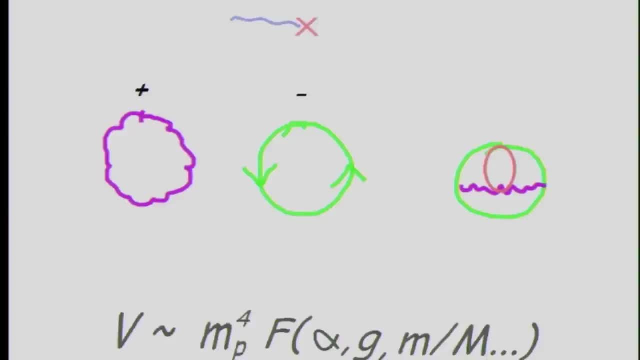 is infinite. how do you actually make some sort of systematic calculation? well, to make a calculation, you have to regulate the theory, cut it off, introduce into the integrals that go around these loops here. oh, incidentally, one important thing here is that bosons contribute positively to the vacuum energy. 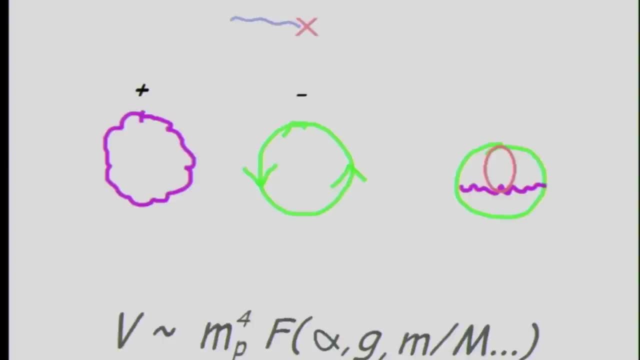 fermions contribute negatively and in general, mixed diagrams of arbitrary complexity may be positive or negative. if you cut the theory off, if you said the end of the integrations occur at the largest mass scale that we know makes sense, namely somewheres around the planck scale, 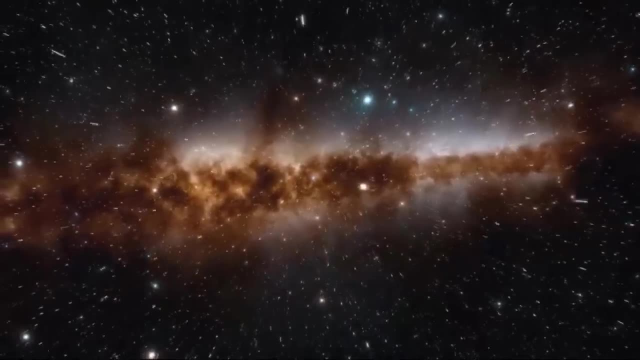 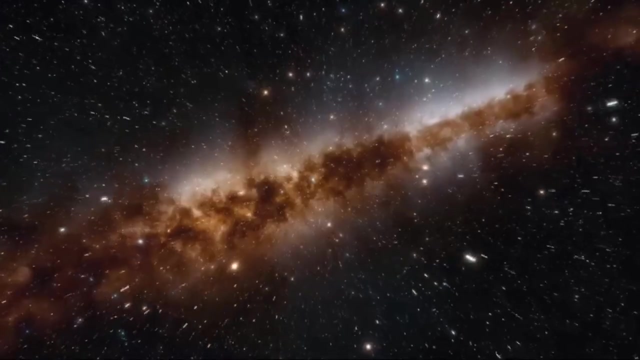 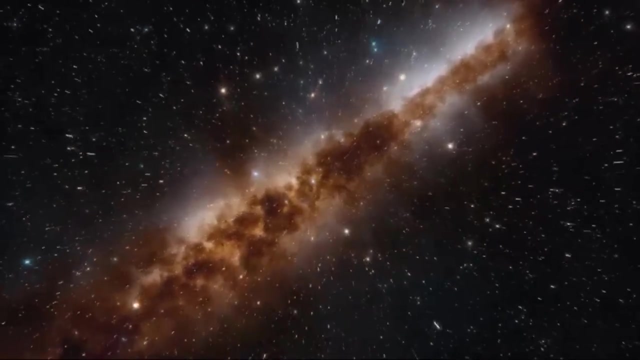 and you don't have to believe that that's a theorist prejudice- then you would find that the vacuum energy, it's cortically divergent and therefore it's order, the cut off to the fourth power times, some function of the coupling constants, whatever they happen to be. 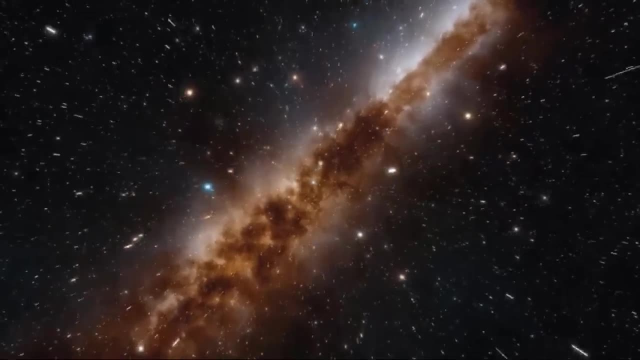 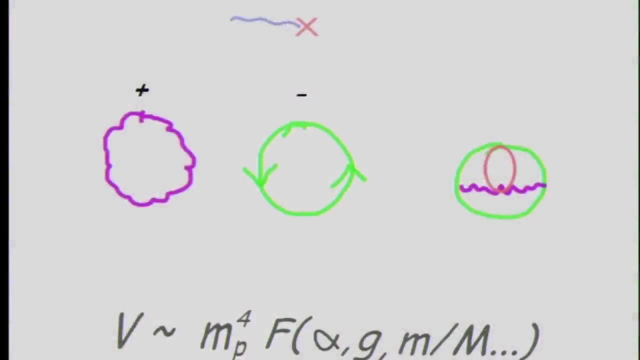 mass ratios, dimensionless quantities. this function begins with the number one in perturbation theory. just these diagrams here, pluses and minuses, of course, for bosons and fermions, and therefore the expected answer. not expected not by observation, but by expected by a theorist who knew no better. 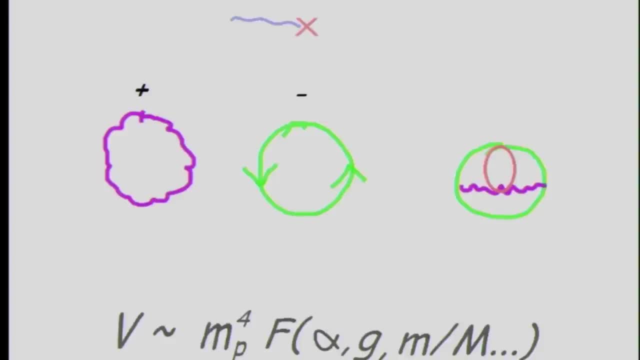 and just made this calculation, would be, of order, the fourth power of the planck mass, and of course that's an absurdly large number. what it would mean is that the time constant for the exponential expansion of the universe would be about ten to the minus forty two seconds. 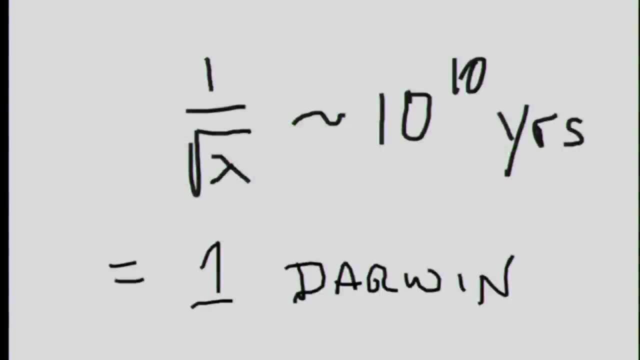 okay universe doubles every ten to the minus forty two seconds in a pure theorist's world. on the other hand, the observed universe doubles in a scale of order time ten to the tenth years, which i like to call one darwin. i call it a darwin because it's about the time scale. 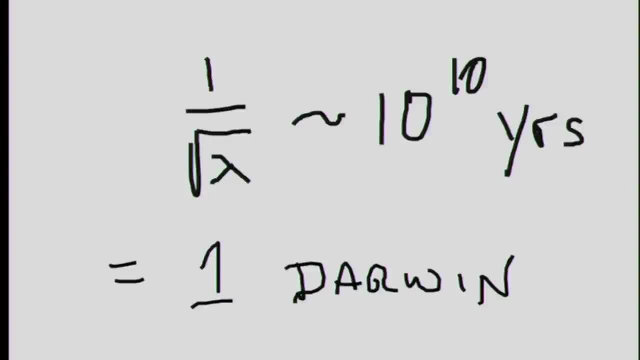 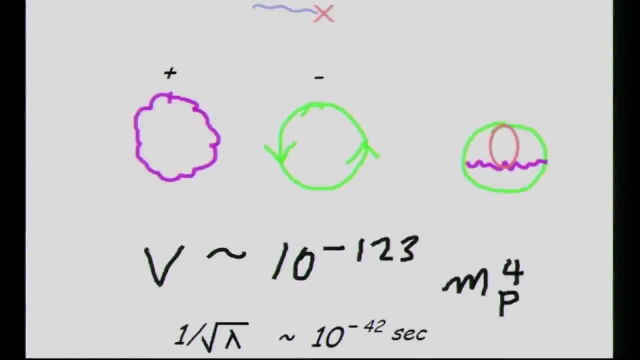 for intelligent astronomers to evolve on the in the universe, and i think it's a good unit of time, a good name for a unit of time, particularly for those people who have anthropic leanings: ten to the tenth years, compared to ten to the minus forty two seconds. 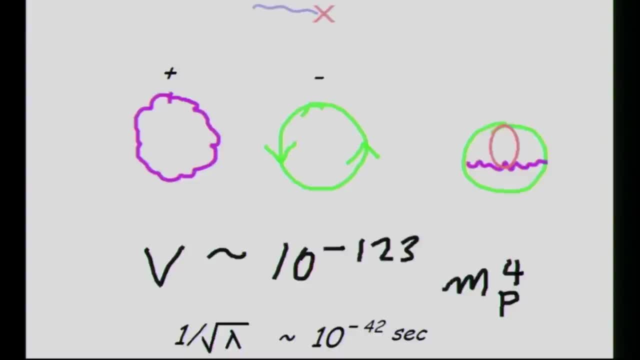 translates into the statement that the vacuum energy is about ten to the minus a hundred and twenty three times m planck to the fourth. in other words, we have a very, very serious fine tuning problem where the sum of all these graphs, each one of which is of order, one times m planck to the fourth. 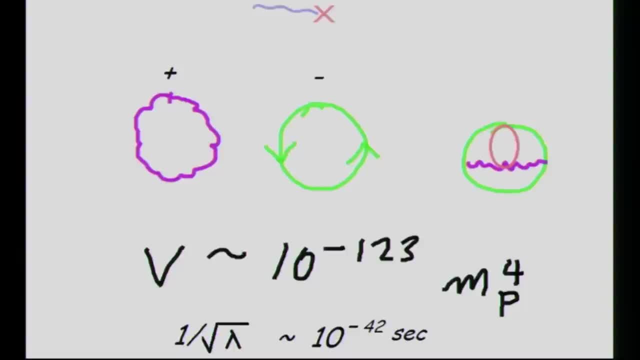 is adding up to something a hundred and twenty three orders of magnitude smaller. one possibility is we're just making a basic mistake. we're not understanding. uh, this is somehow right, except not quite right. the other possibility is question mark. i don't believe this problem can be discussed reasonably. 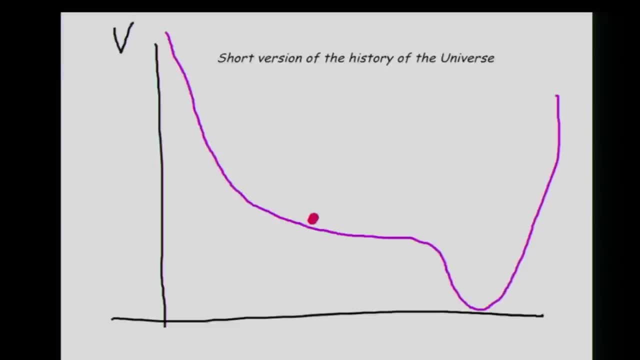 as simply the dark energy problem. i believe it must be discussed in a bigger context. the bigger context to include, i think, the entire history of the universe. and so here's the short form of the history of the universe that will serve us very well. today there is a potential energy function as a function of some field. 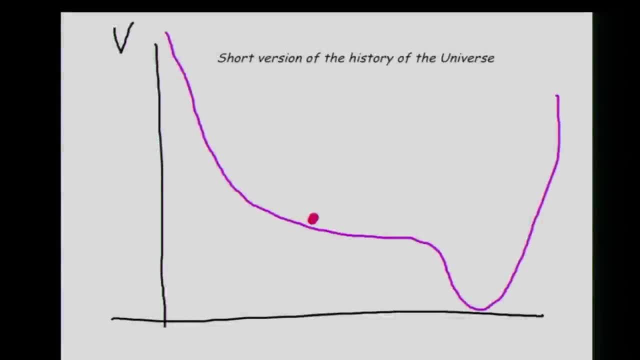 it's the inflationary picture and for reasons unknown this inflationary potential had a flat range over here, pretty flat. the universe slid down, exponentially, expanded along here because the vacuum energy was more or less constant- went over the cliff- the cliff is called reheating- and plunged down to the bottom. 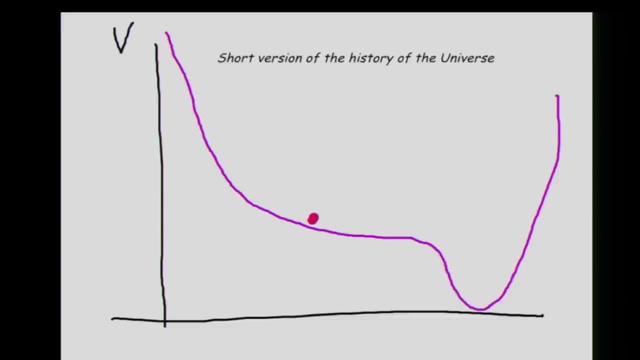 the bottom is not quite at zero energy. it's at this ten to the minus a hundred and twenty three. that's the short form history of the universe and almost everything that we observe. i take it back, just about everything we observe. all occurred either down this slope here or very, very close to the bottom. 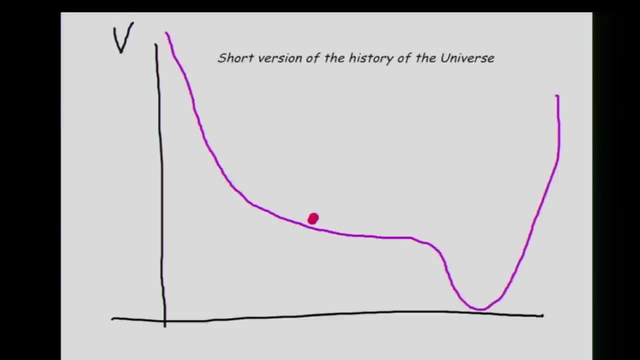 that's the history of the universe in a nutshell: two periods of exponential expansion, one with a time constant of for inflation. it's about- possibly about ten to the minus thirty two seconds down here- ten to the tenth years. i think that's the context we should think about it in. 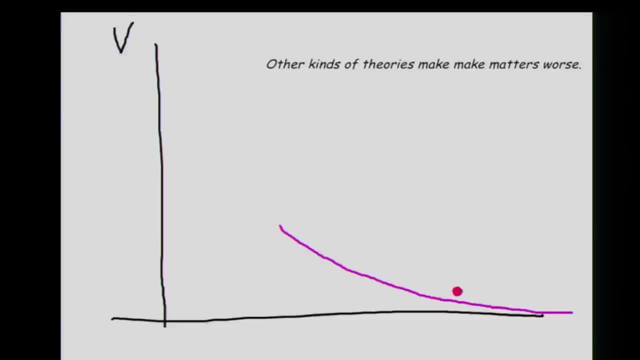 there are other possible explanations of accelerated expansion. one of them is called quintessence. i hate it. i dislike it intensely, but nevertheless we should think about it. it's the idea that the potential doesn't have a minimum. it just slowly slides down to zero. and we're on this very, very slow roll here. 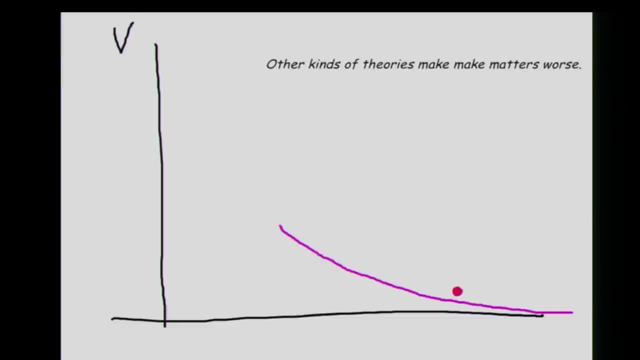 the problem with this is, i think, it just exacerbates the problems. first of all, it still requires you to understand why. at the minimum, it's extremely small, either zero or smaller than ten to the minus a hundred and twenty three. but on top of that it requires a whole bunch of derivatives of the potential to be absurdly small. 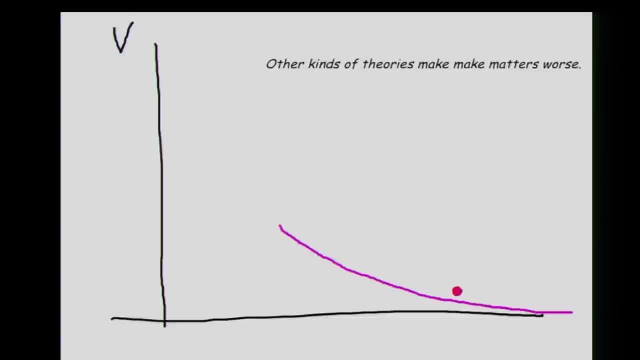 it doesn't seem to do anything positive for you. it just makes matters worse. the fine tuning problem for this kind of quintessence potential is worse than for a single cosmological constant. however, i certainly think we should keep our minds open and ask what it implies. 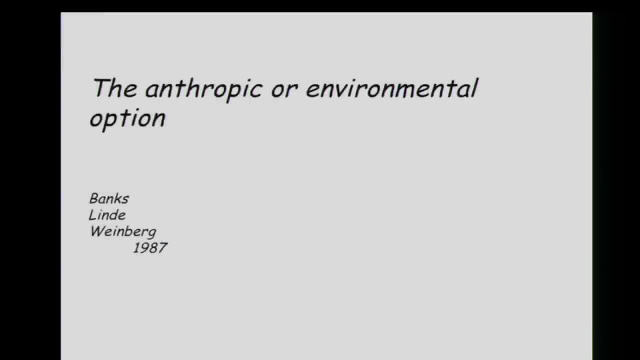 nevertheless, i will not speak about it further, alright, so what is the option on the table? the option on the table is the anthropic option. the idea that the cosmological constant might be determined by anthropic considerations to my knowledge first appeared in papers of banks, linde and weinberg. 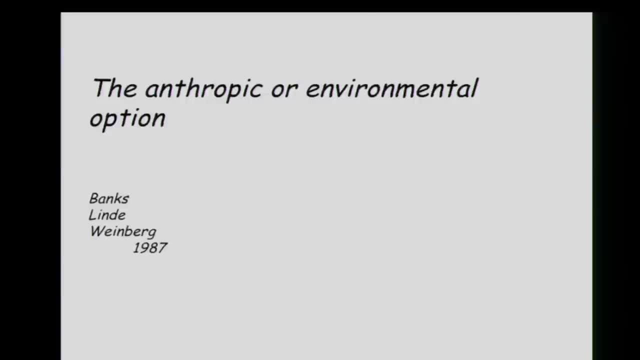 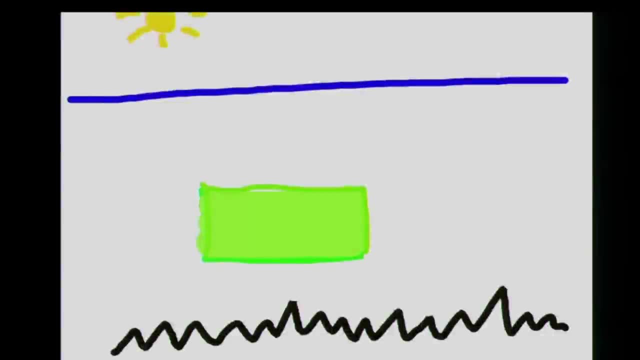 this is not one paper. this is three different papers and they all had pretty similar ideas. weinberg's idea was more quantitative, but let me give you a metaphor for it, a metaphor for what the idea is. i think the metaphor is useful, particularly for people who are not deeply ingrained in the mathematics of inflation and so forth. 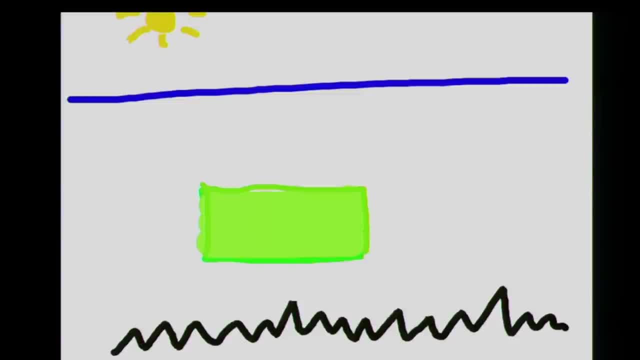 here's an analogy: here's the sea, here's the sun, and this thing here is a submarine. we live in a submarine. we live in a submarine and the green submarine is a rather marvelous submarine. the bottom of the sea is a very dangerous place for the submarine. 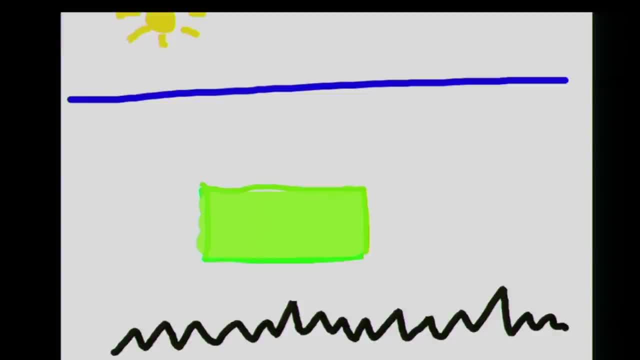 it will get crushed. the top of the sea also happens to be dangerous. it will get fried by the sunlight, made of some sort of material that gets fried by sunlight. people are in it and they notice that they've been floating midway between the top and the bottom for a very long time. 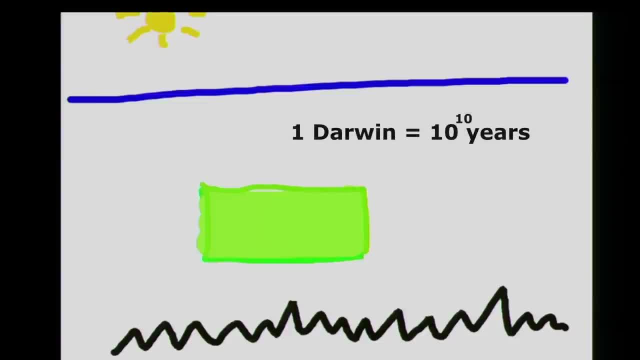 how long a darwin. they've after all evolved. they've evolved enough to ask questions. they've been floating in the middle for a darwin. on the other hand, this submarine is made of all sorts of stuff: carbon, silicon, iron, other stuff with a very different density than water. 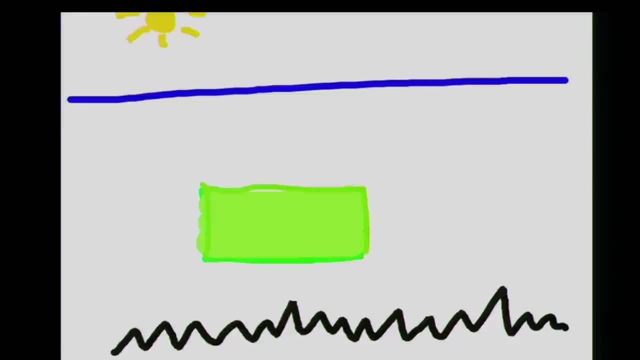 some of it is lighter than water, some of it is heavier than water. by what miracle is it that this submarine just managed to float halfway in between for 10 to the 10th years? that's the miracle that they discover, if it's just a tiny bit too heavy. 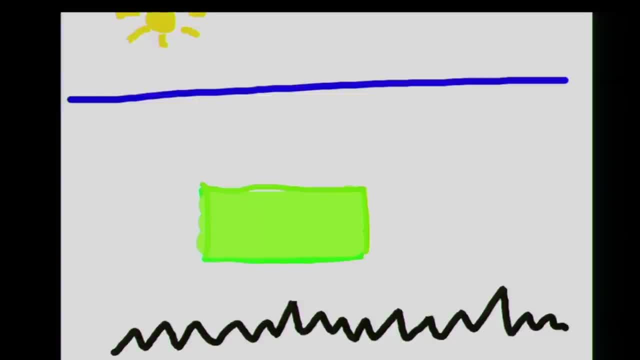 if the composition is just slightly wrong, they fall. if the composition is slightly wrong in the other direction, they rise. what's going on, they ask themselves. well, some- either smart or perhaps stupid theoretical cosmologists, physicists, come along and say: ah, we know what this means. 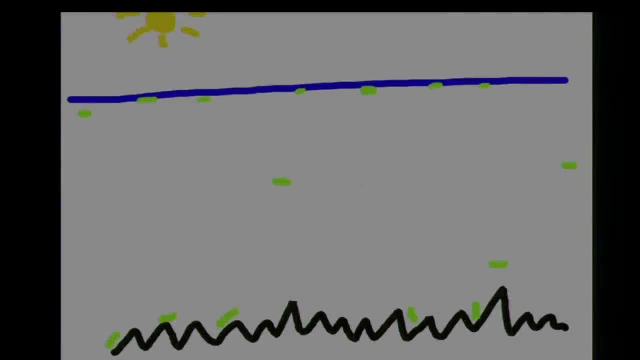 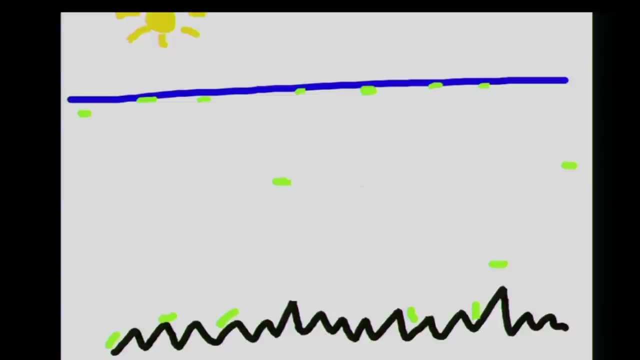 is. there's just a hell of a lot of submarines out there. there's a lot of submarines, all of slightly different composition. most of them, in 15 seconds, fell to the bottom of the sea or rose to the top. nobody in those submarines. they're completely empty. 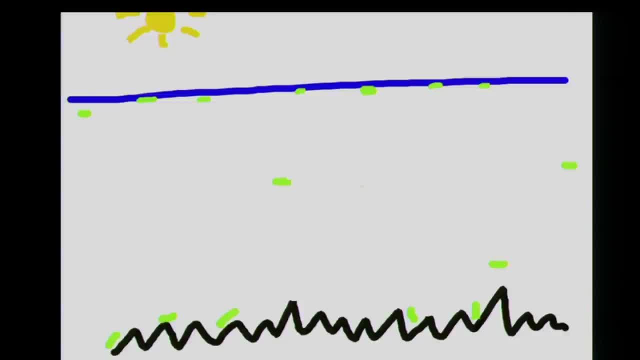 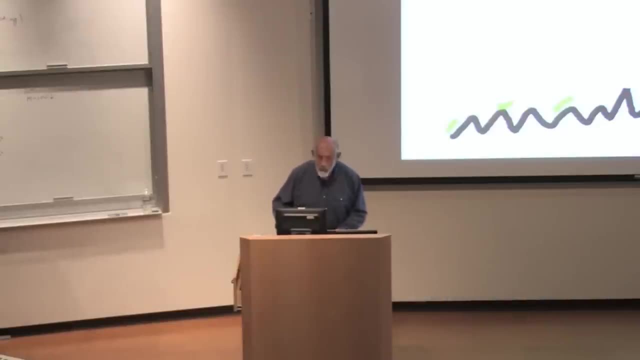 a handful of them lasted for an hour. nobody in them either. some tiny, tiny, tiny fraction of them was of composition, accidentally, just right to be able to float in the middle. those are the ones that have astronomers. that's the logic, if you like, that's the logic of anthropic reasoning. 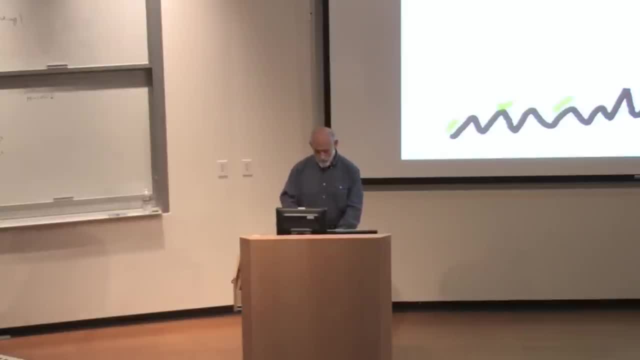 it's no more philosophical, it's no deeper than that. that's the idea, is it right? that's for us to test, both theoretically and experimentally. alright, what is the sea in which we all float? let's call it the sitter space. 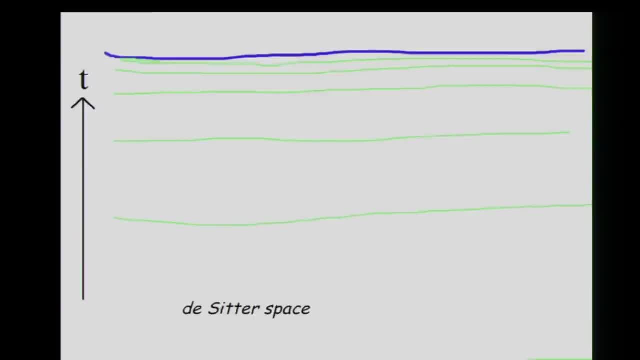 and let me remind you what the sitter space is. this: the sitter space is a generic. the sitter space it's not necessarily the world that we live in today, it's not necessarily the world of early inflation. it's just a generic: the sitter space. 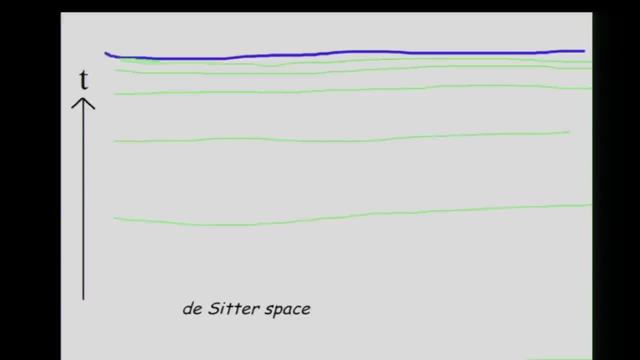 a generic. the sitter space is an exponentially expanding space and it can be drawn on what is called a conformal or a Penrose diagram. it's infinite in extent, in time extent, but to draw it in a way that guarantees that light rays move on 45 degree angles. 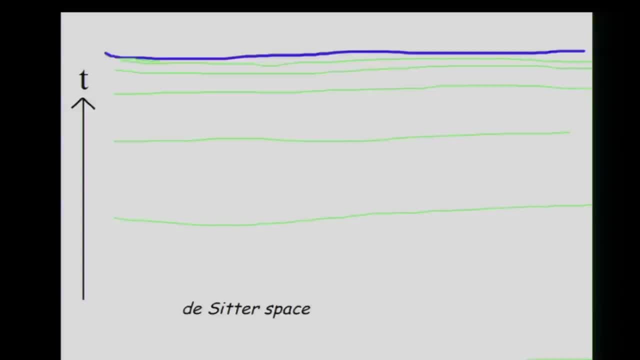 you have to draw it as if time came to an end. the sequence of green lines here are time slices. this is t0, t1, t equals 2, t equals 3, t equals 4. there's an infinite amount of time, but the causal structure. 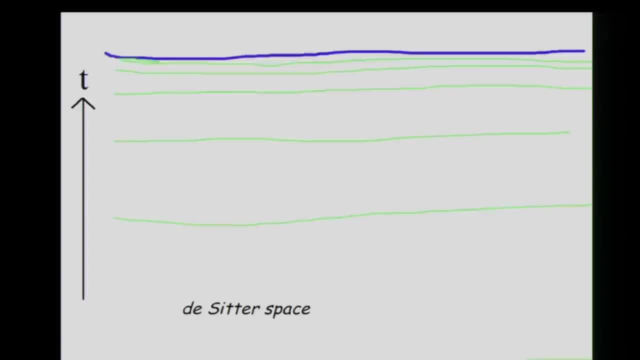 the geometric structure is such that it's best drawn in this way here. so let me show you what that does for you. if you draw it in this way, you can immediately see why there are horizons, why the sitter space has horizons. two observers- vertical lines- are observers in this world. 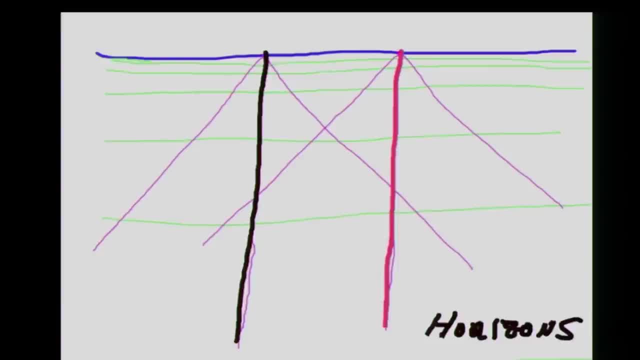 and they can look back, and they look back at any given time along their light cones. here they are two of them. at some time in the past, in fact, their past light cones overlapped. they can see each other rather easily. in fact, any observer up here can see his friend. 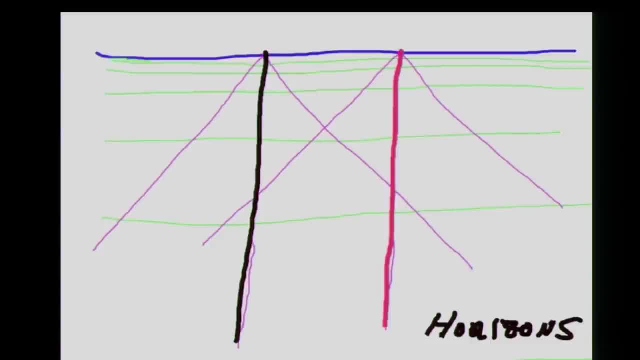 in the sufficient past, but what he can't see after a point, he can't see his friend at the same time. there is an event horizon. this is the black person's event horizon. this is the red person's event horizon. the black person cannot see outside his own light cone. 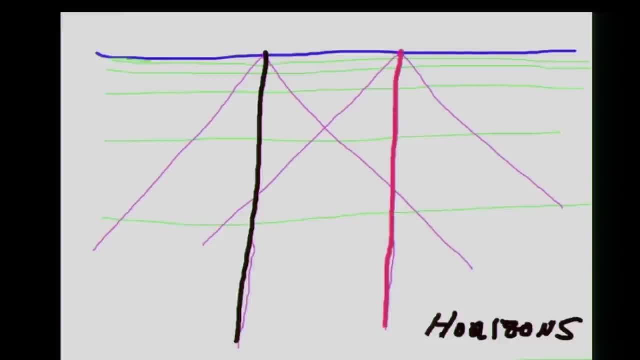 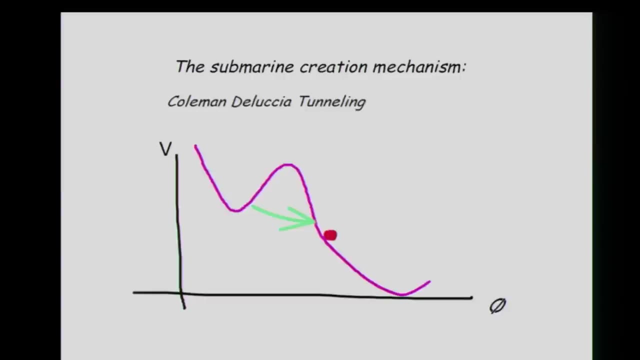 the red person cannot see outside his light cone. those are event horizons, and this is one of the reasons that it's useful to draw the sitter space. in this way, you see everything that's going on on a single map. okay, that's the background, that's the sea that we live in. 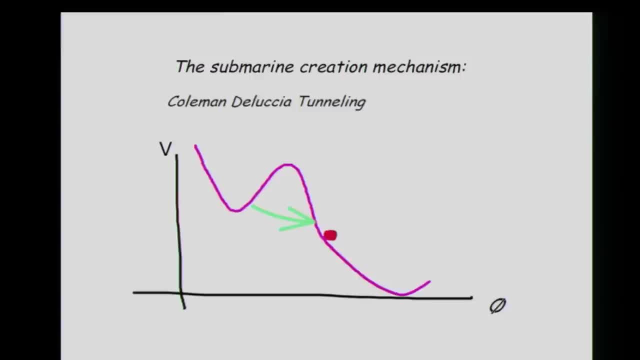 or at least according to a hypothesis. that's the sea that we live in, not necessarily the 10 to the 10th years or the 10 to the minus 42 years, but some sea like that. and the question is, what is the submarine creation mechanism? 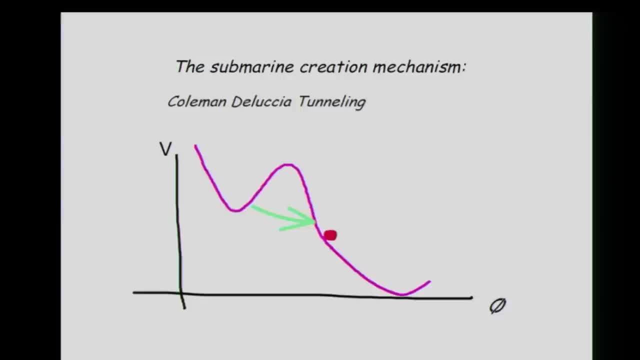 the submarine creation mechanism is the mechanism that creates pockets of space that we can live in. the hypothesis that that most theorists who think about this think of is Coleman de Lucha tunneling. I will explain that in a moment. but let's come back to a scalar potential. 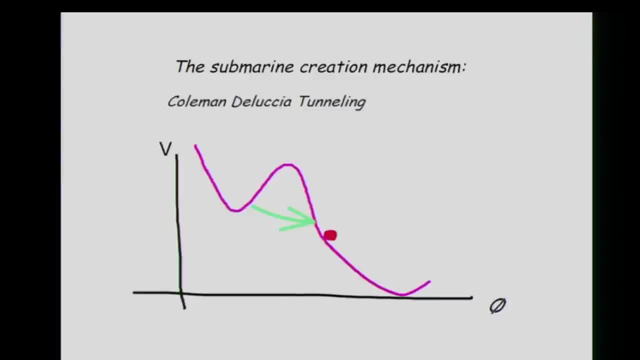 if there's a scalar potential and it happens to have sufficient structure with sufficient number of minima- a generic function with lots of minima, or something like that- then tunneling is possible- tunneling from one minima to another. this is a picture of what tunneling would look like. 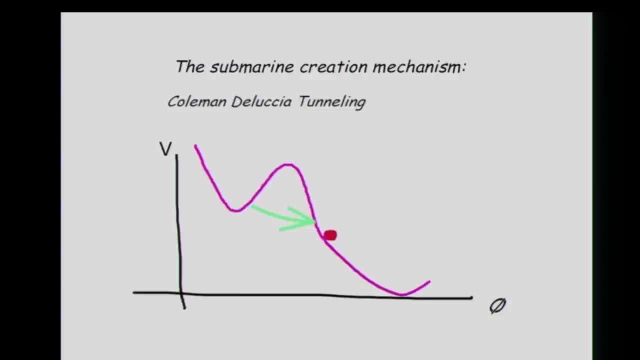 for a Coleman de Lucha instanton, you tunnel from one minimum out of that minimum and then typically roll down to the next minimum. that's the structure of Coleman de Lucha instantons, and I've drawn here a very generic kind of roll down. that is what one would expect. 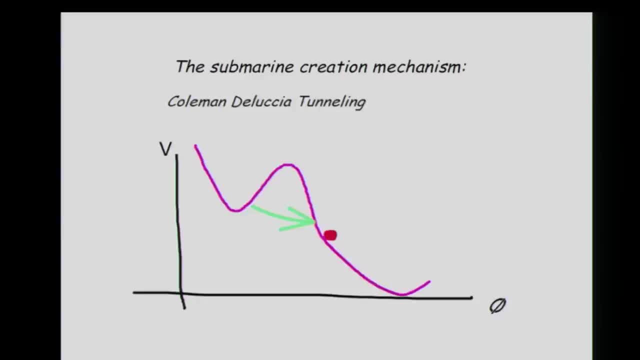 from a generic function with a single extra minimum in it, two minima. what kind of cosmology does this lead to? by that I mean, what kind of cosmology does this lead to in the submarine? the submarine is a bubble. the submarine is a bubble that nucleates. 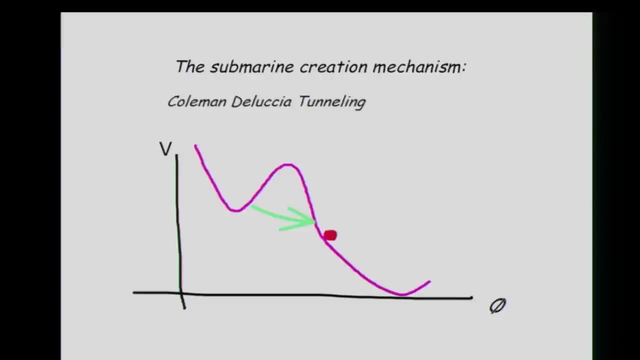 when this tunneling event happens. the tunneling event is a local event, a small little event which nucleates a bubble. these are the bubble walls. the bubble walls spread out just like the bubbles of gas in a super cooled fluid. the bubble spreads out and the interior of the bubble 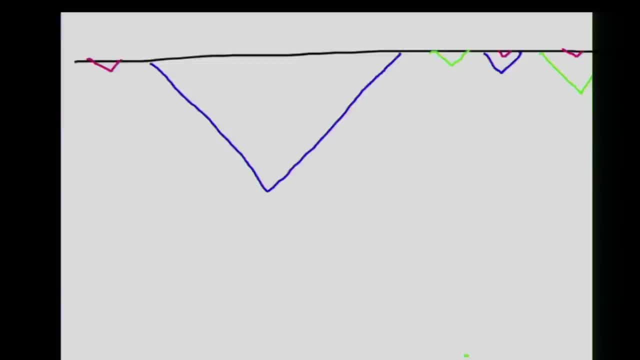 is a new environment, the new environment on the other side of the potential. the question is: is this a good submarine? there are many of them. it keeps happening all over the place, so there are lots of them, many, many different types, if physicist speculations are correct. 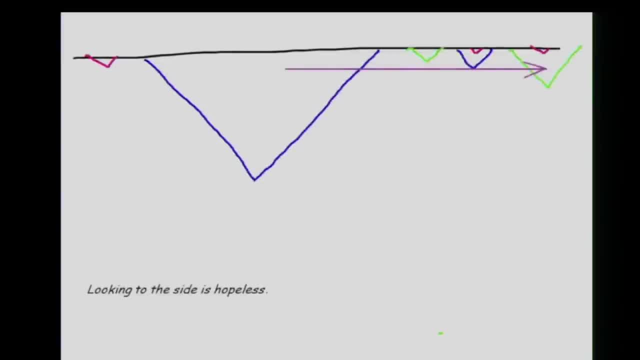 the question we want to answer is what phenomenological experimental observational signals can confirm this. unfortunately, the list is very, very limited. I know of only one or two, and even those would take a great deal of luck to be able to observe. but let's begin. the first thing is looking to the side. 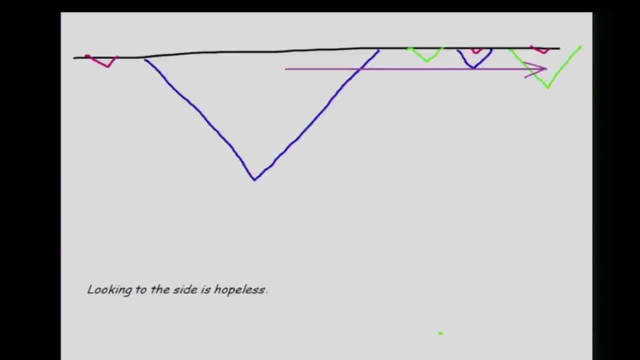 trying to see these other bubbles is hopeless. if we live over here, our horizon precludes us seeing them, period. they are simply outside of our horizon. we cannot see them. so looking to the side, meaning to say looking for other bubbles, similar bubbles, is out of the question. 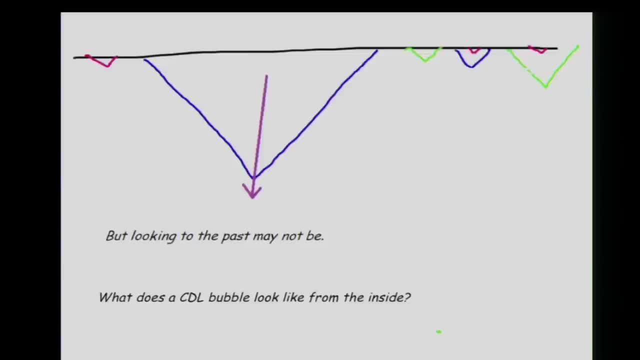 what is possible is looking back in time to try to discover whether there is any evidence of a bubble nucleation that we were born. looking into the past and trying to see our origins in a bubble nucleation may not be impossible. so the question is: what does a bubble look like? 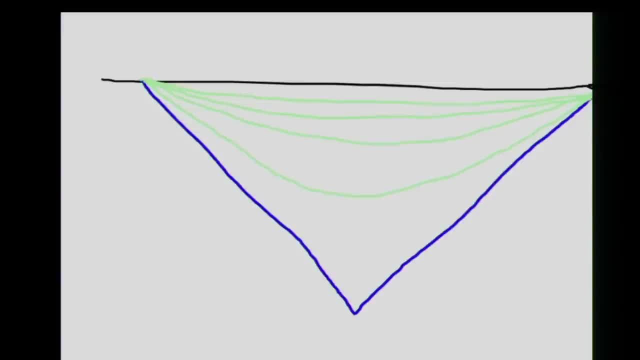 from the inside. here's a picture of it again, but now I've drawn in some surfaces of constant energy density, surfaces that you could think of, and should think of, as slices of constant time, not for this all over external sea, but for the observer on the inside. 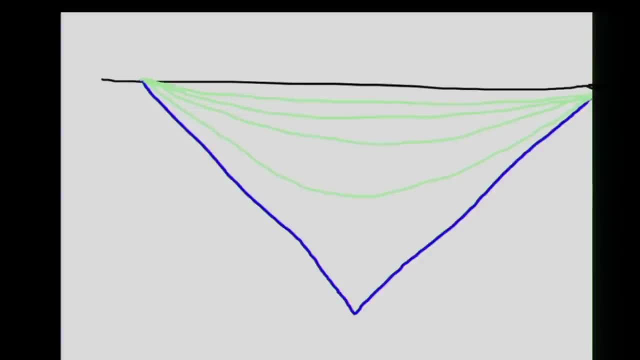 this takes a little bit of mathematical study to find out what the surfaces of constant energy density look like, but they look like this. what kind of geometry- spatial geometry does the observer on the inside see? this would be a slice of space. the answer is they see negative spatial. 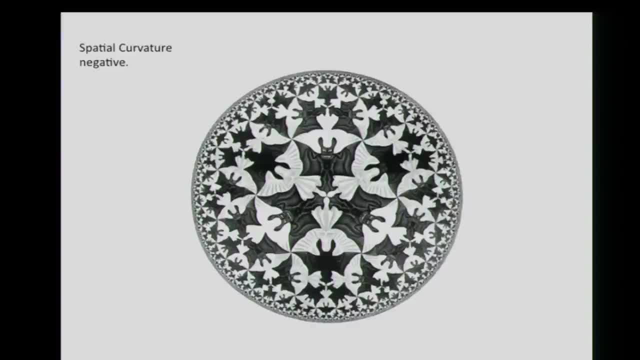 they see an infinite universe. let's go back, going from here out to the edges over here on one instant of time is basically moving on a geometry which looks like I think you've probably seen this before. this is just basically a picture of a negatively curved, uniformly negatively curved. 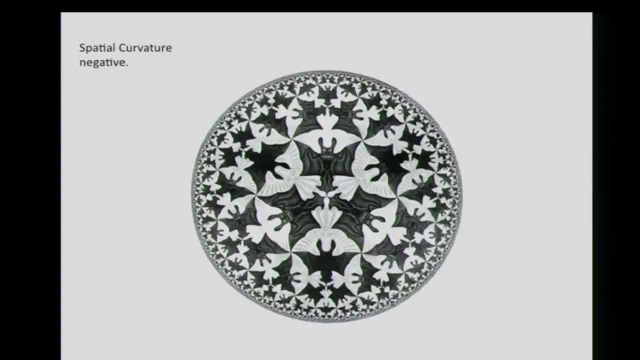 it's called the Poincaré disk and it's just a picture of negatively curved space on the boundary. the space is infinite. the space is infinite even though it's a bubble contained in what looks like a finite region. the space itself is infinite and it's negatively curved. 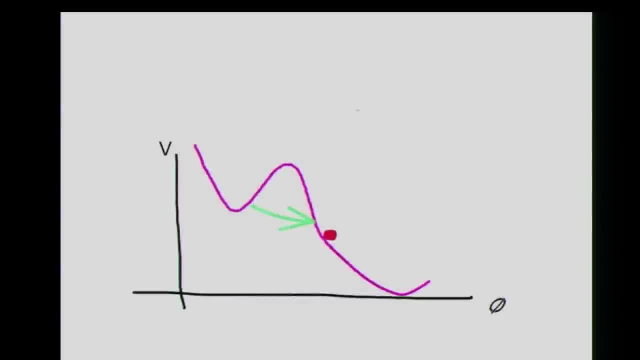 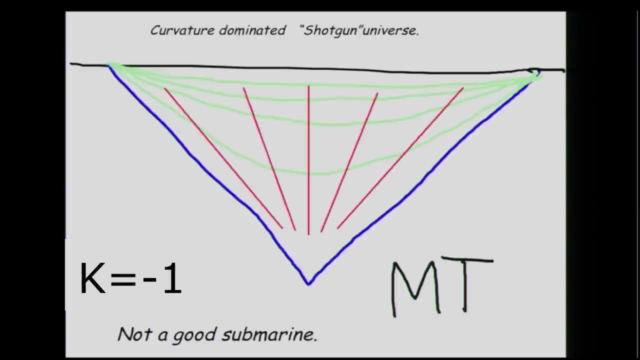 okay, let's go back for a moment and ask now again a little more about what this bubble looks like. here again, I've redrawn the picture of bubble nucleation with a generic potential. a universe born in this way could be called a shotgun universe. it's, first of all. 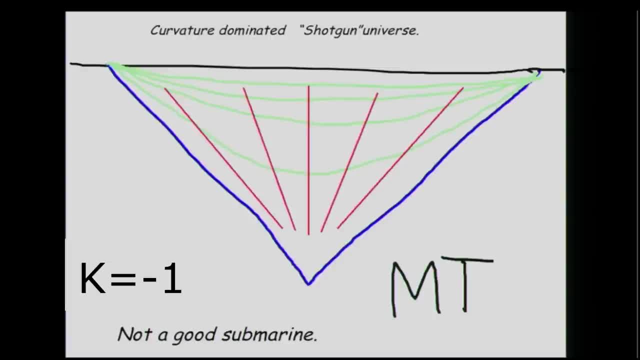 curvature dominated. it has a lot of negative curvature in the early period and negative curvature means that the stuff which is shot out is above the escape velocity- escape velocity for forming galaxies in particular. it's shot out, diluted very fast, it's empty and it's k equals minus one. 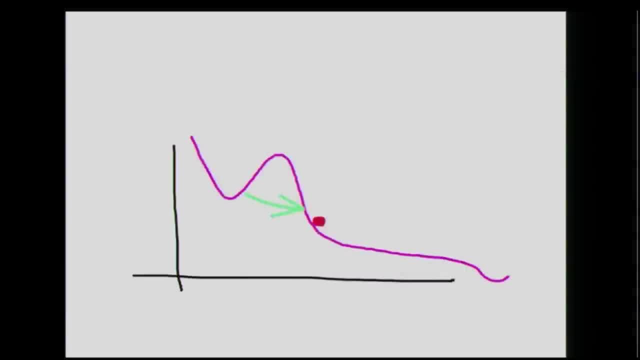 it's not a good submarine. what do you need to make it a good submarine? you need a period of slow roll inflation to dilute the curvature. if you dilute the curvature during some period of slow roll inflation, then the production of matter is different. everything is produced. 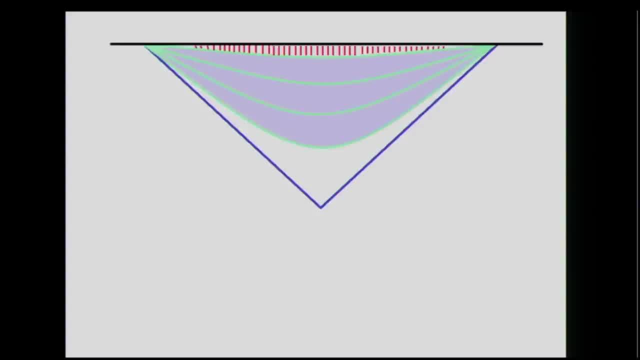 more or less at rest with respect to each other and there's plenty of opportunity for um. okay, how much inflation do you need in order to create an acceptable submarine? that is the anthropic bound on the amount of inflation that you need, if you take the observational bound. 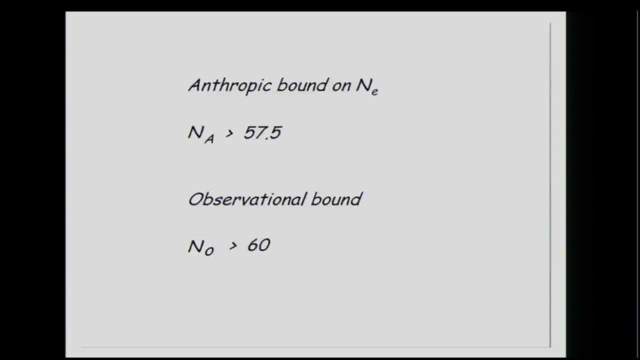 on the number of e-foldings to be 60. now, of course, 60 is an arbitrary number. it could be 30, it could be 40, it could be 50, depending on the model. but if you take a model in which the observed bound 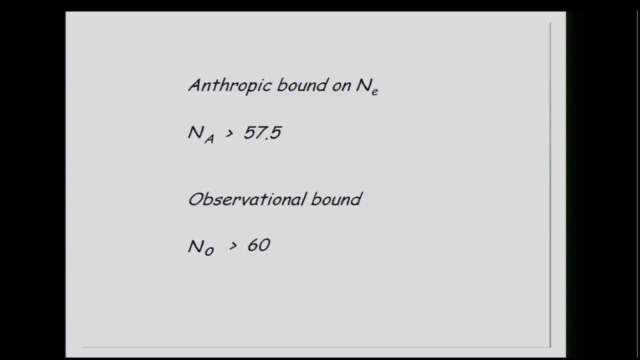 the number of e-foldings is greater than 60, what it says is that the anthropic bound is greater than 57.5. now, the actual invariant number is the difference between the observed bound and the anthropic bound, and what it says is that the anthropic bound 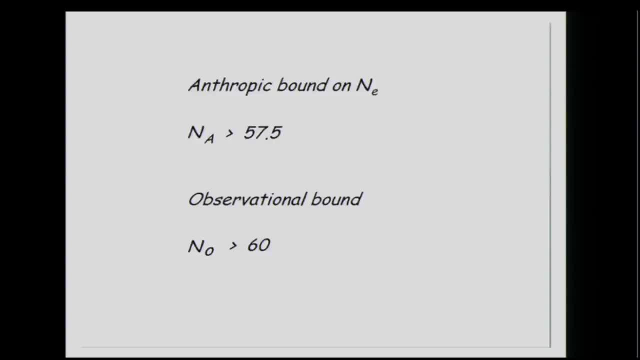 is rather close to the observed bound, in other words, that if the number of e-foldings was much less than 60 in this model, we wouldn't be here. it doesn't say that the number of e-foldings is greater than 60. alright, here is a. 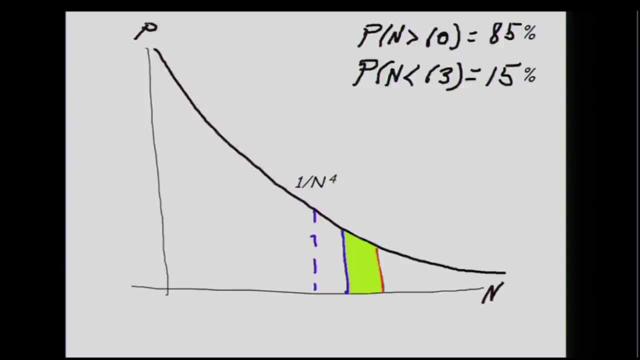 typical picture. it's hard to make a lot of e-foldings. you have to tune parameters, you have to make that potential very flat. if you just take a random sampling in parameter space, you'll find out that the probability for a given number of e-foldings tends to fall rapidly. 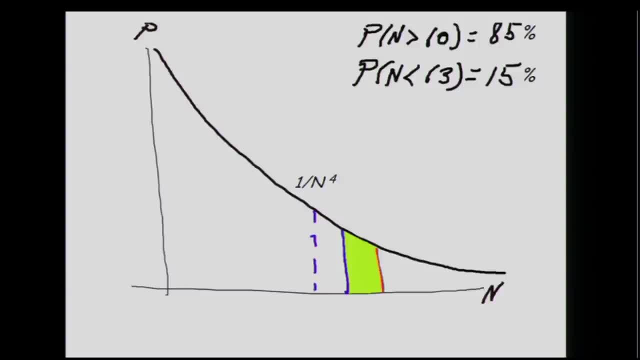 just because it takes more and more fine tuning to make a lot of e-foldings, and in one simple model, one simple statistical model, the probability for n e-foldings falls like one over n to the fourth. it's just hard to make them. so here's a picture now. 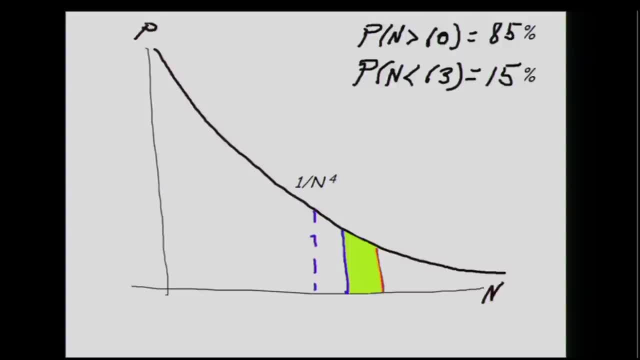 here is the anthropic bound of 57.5, here's the observed bound of 60, and if you ask the question, not what's the probability that you have more than 60 e-foldings, but what's the probability that you have more than 60 e-foldings? 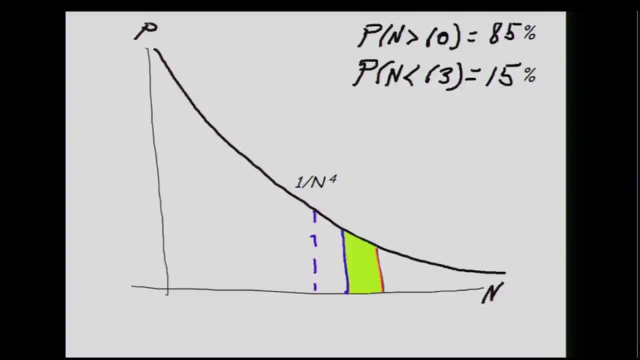 given that you have more than the anthropic bound, what's the probability that you have more than 60? given that you have more than 57.5, then the answer is about 85%. alright, so the point is that anthropics, if you like, is the explanation of why there was a long 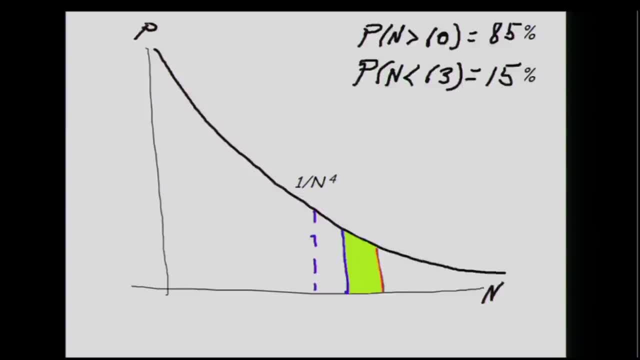 period of slow-roll inflation. on the other hand, you could also ask what's the probability that we have a chance that the number of e-foldings is low enough that we can see back more or less of a bubble nucleation, event that would require that the number of e-foldings 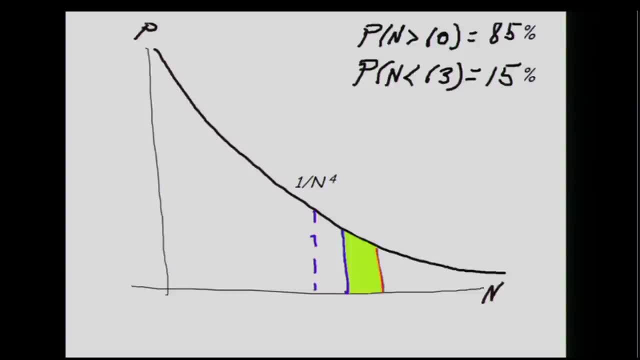 was no bigger than about 63, more than 63, everything gets diluted away and if you use the same parameterization, you find out that it's about 15%. now, there's nothing hard about that number, it's just a model. but 15% is a small number. 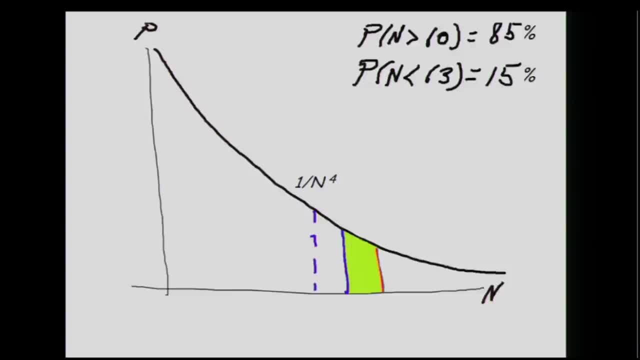 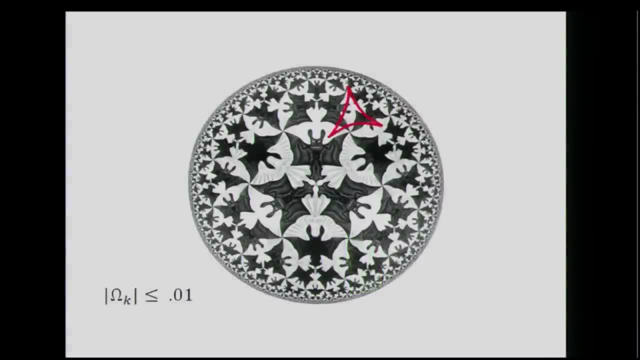 it's a long shot, but it's not absurdly small. if we are very lucky in this region here and then we can see back. what do we see? the first thing we would see is negative curvature. if this theory is right, that's the most robust prediction. 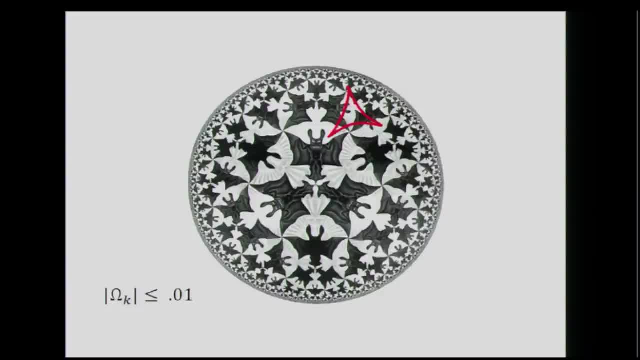 of bubble nucleation. now I would say the most robust prediction is not that you see negative curvature, but that you don't see positive curvature. if we were to see positive curvature in the next round of curvature experiments, or the next two rounds, we would have to go back to the drawing board. 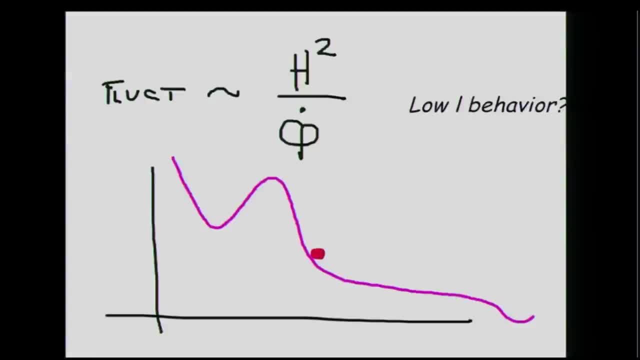 on this idea. another thing is about the fluctuation spectrum of density perturbations. the fluctuation of density perturbations, well known formula, you probably mostly know it. the power spectrum is proportional to this- is V. this is the vacuum energy divided by the rate of 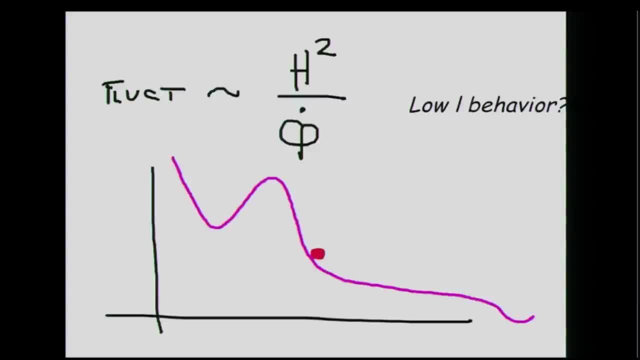 the velocity as you fall down the hill here and as you come off this hill. here two things are true: h squared is bigger than it would be a little bit later on the flat portion and phi dot is bigger in general if you look at reasonable parametrizations. 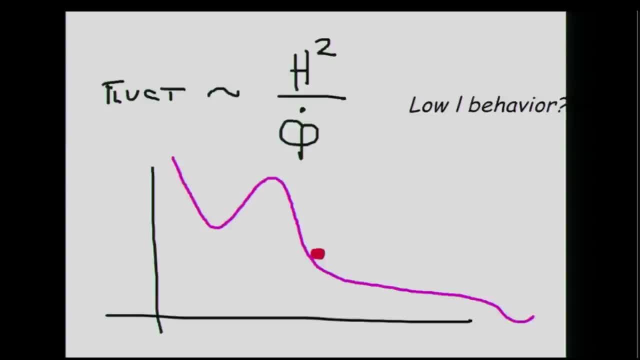 it looks like phi dot tends to win and the effect is that the fluctuation spectrum at the very beginning of the slow roll here is suppressed. now it could be enhanced, but I think the best bet is that it's suppressed or low L suppression due to the fact that you're riding. 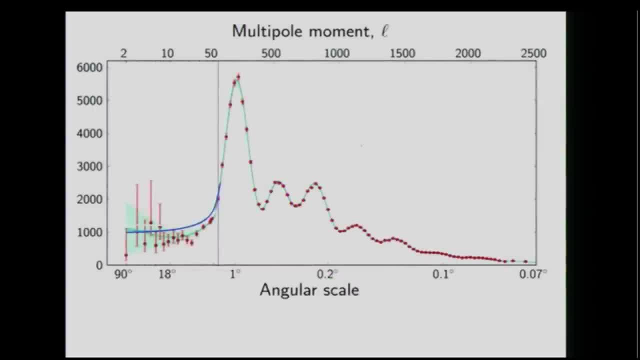 down a hill here. this is a made up picture. I didn't make up this part of the picture. I made up this part of the picture here. I am told that and I cannot confirm this. I am told that there is a low L anomaly where the best fits. 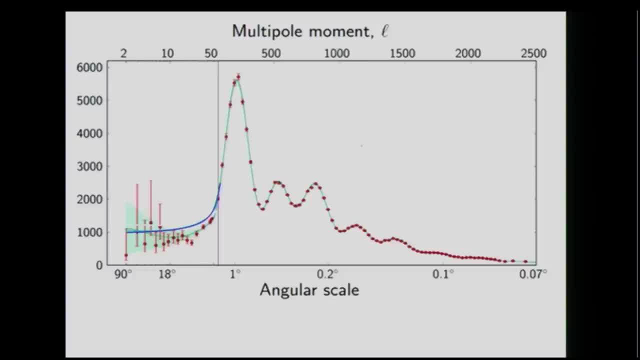 to a generic vanilla flavored slow roll picture would look something like this, where the beta is a little bit low. this, of course, is pi in the sky. this was not after the fact. incidentally, the prediction of a low spectrum is about 10 years old. forget that. 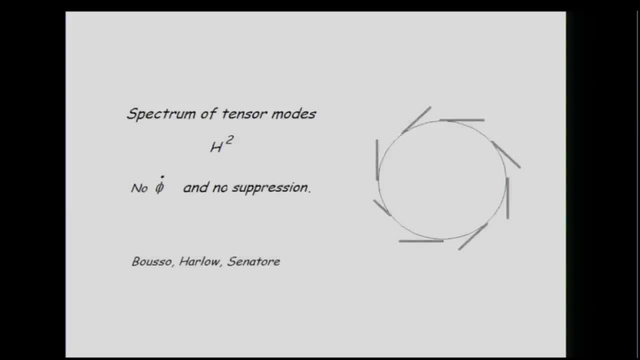 another fact that if you look at tensor modes, tensor modes are proportional. the spectrum is proportional to h squared, with no phi dot in the bottom. this is an observation that is about to come out, I believe, by Busso, Harlow and Senatore, and notice that the formula does not have a phi dot. 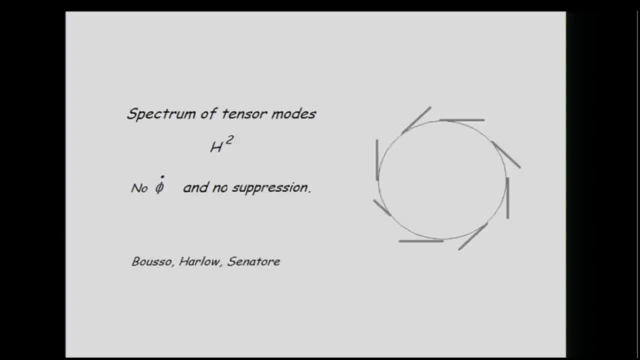 so that if we do see tensor perturbations, they should not be suppressed. in fact one might say that they should be slightly enhanced at early times because h squared is a little bit bigger. so one of the things you might expect if you can see these kind of things. 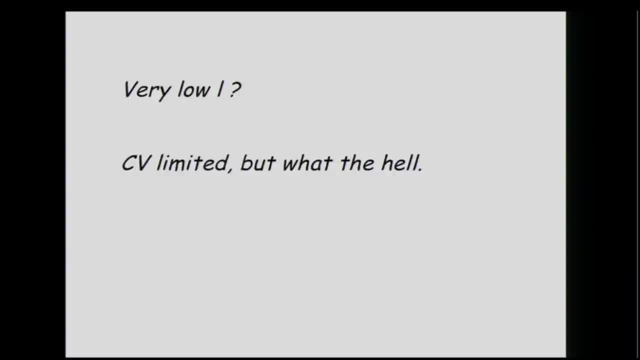 is just such a relative enhancement of the tensor spectrum. finally, what about, incidentally, that phenomena that would take place, an L from 2 to 50? what about extremely low L? well, we know that extremely low L is cosmic variance restricted, but still, let's just go ahead. 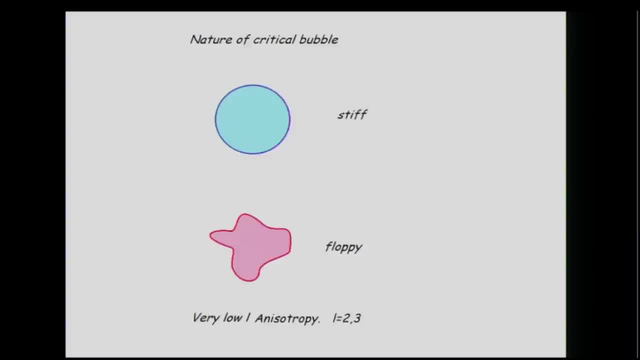 and ask what it has to do with. what very, very low L stuff could have to do with is the nature of the critical bubble that forms at the very beginning. if the critical bubble is stiff, if the parameters are stiff, meaning to say that the surface tension is very much larger than other parameters, 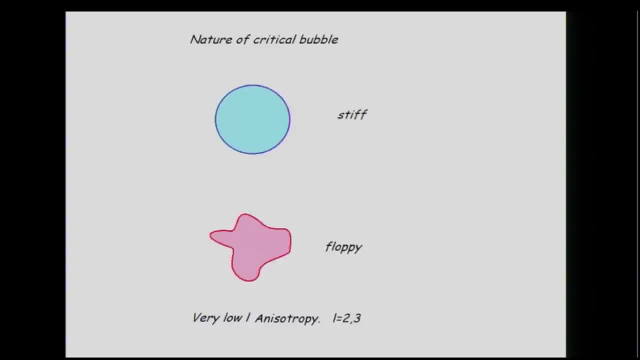 then the bubble will be very spherical. if the surface tension is smaller, the bubble can be floppy. in fact, there's a whole range of floppiness that goes all the way to the possibility of multiple connectedness and really complicated things. this kind of thing could lead to very, very low. 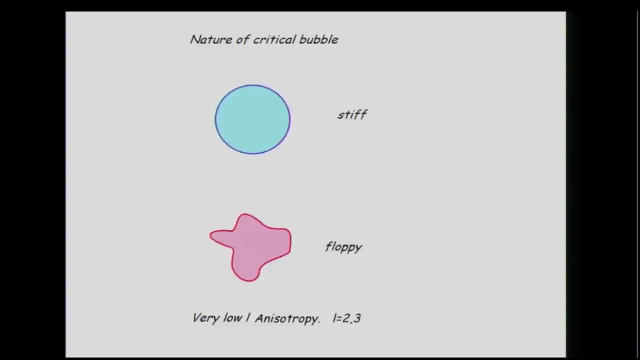 L anisotropy- LOL- means L of 2 or 3. those are all of the signatures that I know of. what should we do? we should keep pushing. we need to know whether W is really equal to minus 1, whether it's a cosmological constant. 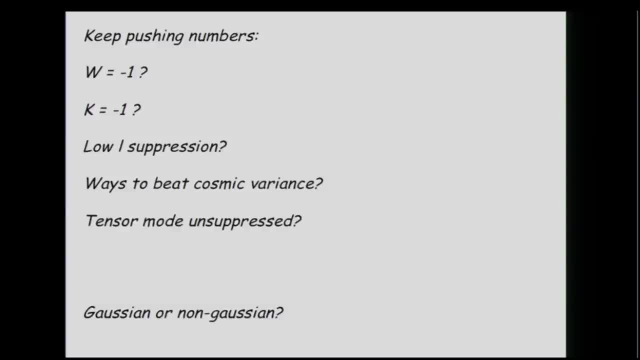 if we can measure the curvature, great. if it comes out to be negative, we're in business. if it comes out to be positive, we go back to the drawing board. is there really low L suppression? well, the only way to find out is to beat back the cosmic variance. 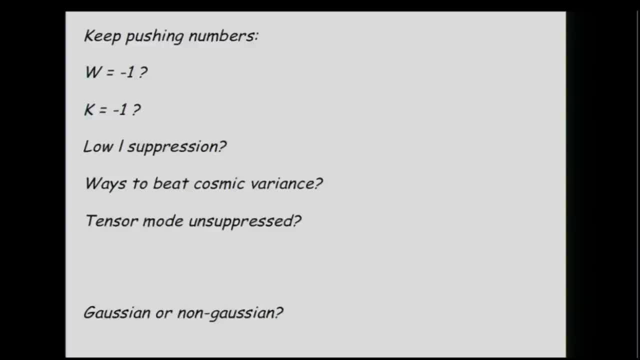 and I'm told that there are ways to try to beat back, but I won't go into them. tensor modes: very important and in particular, are they unsuppressed relative to the scalar modes? finally, there's the question of Gaussian or non-Gaussian, and I haven't mentioned it all. 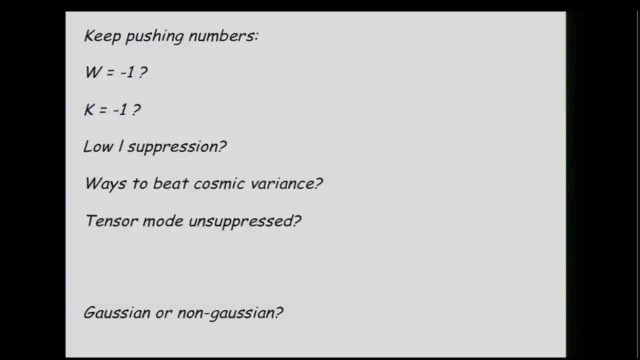 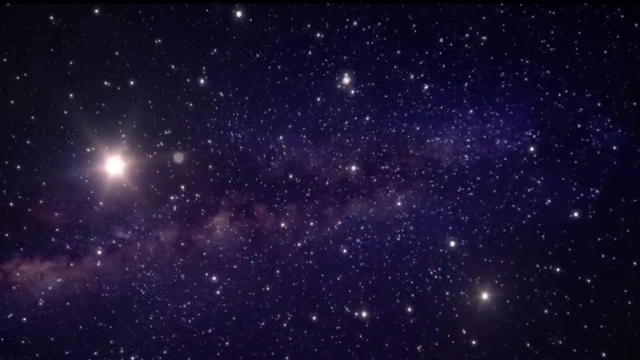 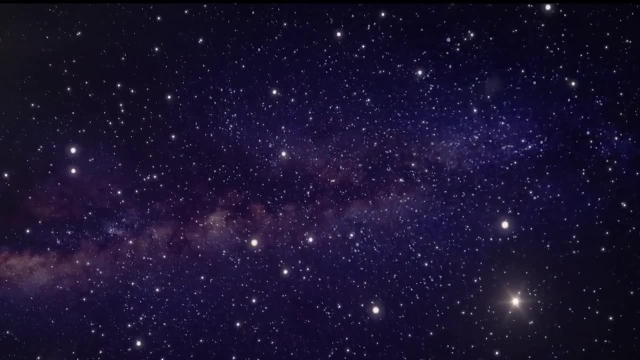 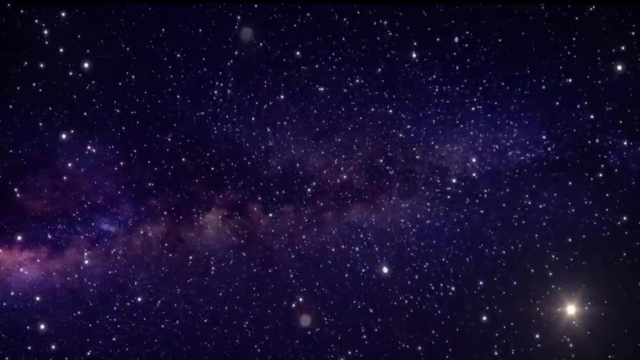 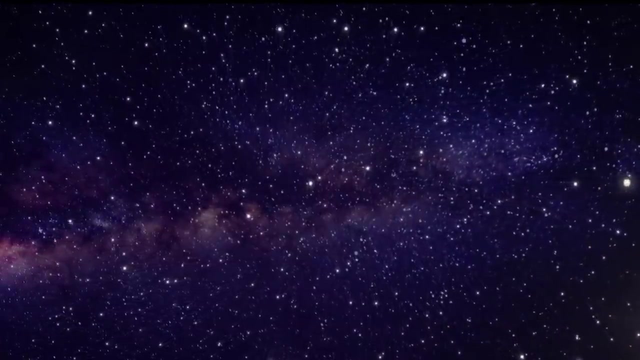 because I don't know how it fits into the story altogether, and thank you very much for watching. see you next time. bye.